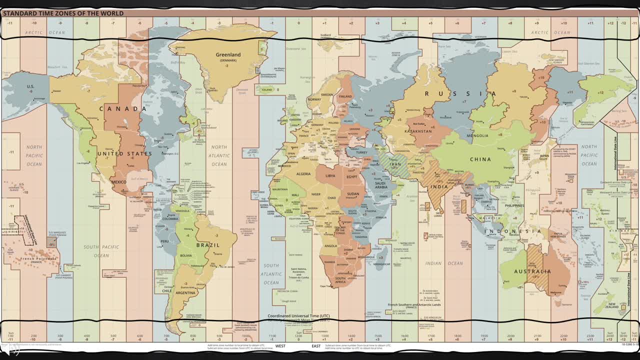 So different countries follow different time zones or UTC. So different countries have different time zones or UTC. If you look at the Philippines, we are on the Plus-8 UTC. If you look at the Philippines, we are on the Plus-8 UTC. 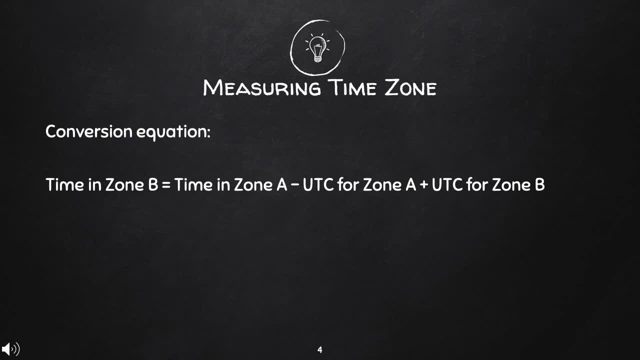 How do you measure time zones of different countries? So we have here a conversion equation: Time in zone B equals time in zone A minus UTC. Time in Zone B equals time in Zone A minus UTC. us UTC for zone A plus UTC for zone B. This can be quite confusing, so I will. 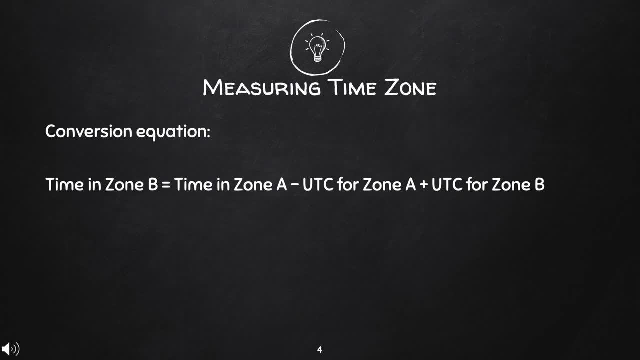 show you two examples on how to measure the time zones. For our first example, what time is it in Los Angeles PST UTC offset negative 08? when New York Stock Exchange opens at 930 PST negative 05? so just remember the UTC of set for each. 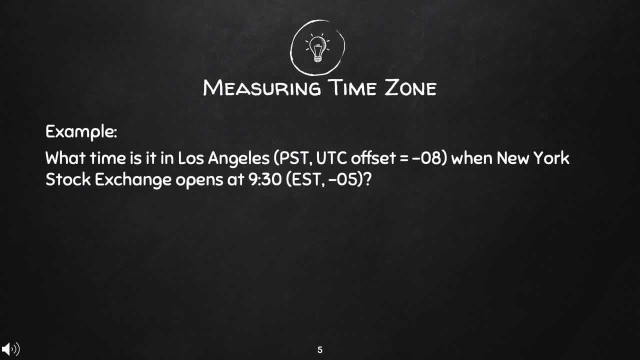 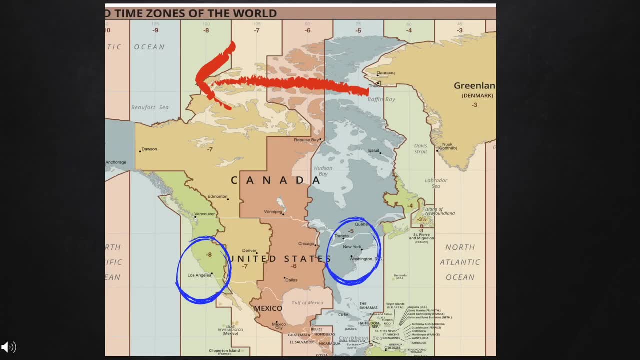 place, plus Angeles, which is negative 08, and New York, which is negative 0, 5. let us find New York and Los Angeles in the map. so this is a bigger version of a map. encircled in blue are Los Angeles on the left and New. 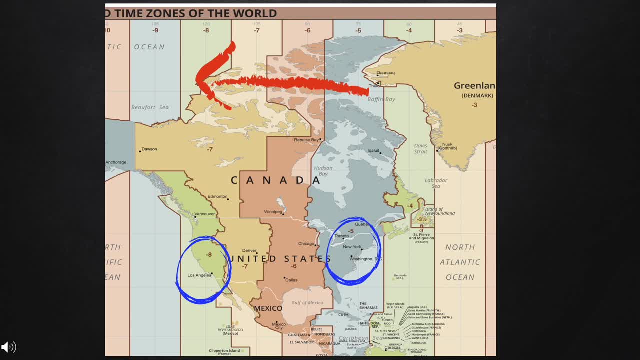 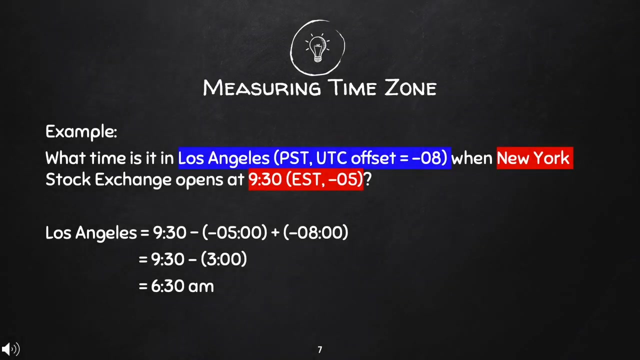 York on the right. so Los Angeles is negative 8 and New York is negative 5. since we will find the time for Los Angeles as compared to New York, we will solve this as going to the left. so look at the red arrow when solving or converting towards the left. you subtract the UTC offsets. what did I mean by? 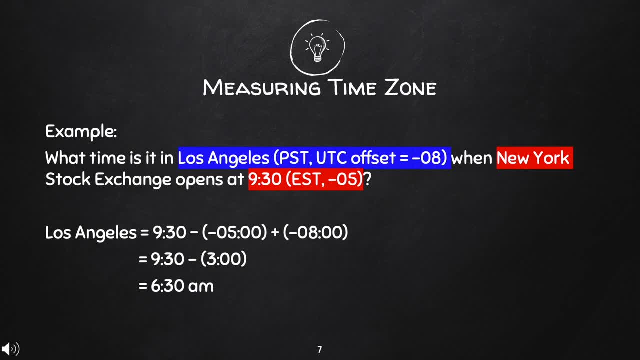 subtracting the UTC offsets. observe the UTC offsets problem again. highlighted in blue is Los Angeles and highlighted in red is New York. so the formula here is Los Angeles equals. then we will write the time for zone a, which is 930, New York. that's 930 minus open, close parenthesis, negative 5. 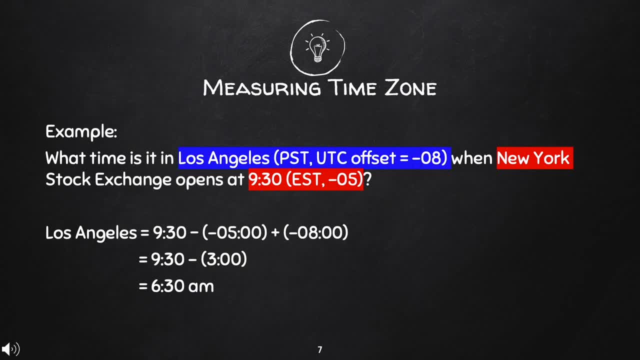 the UTC offset for New York plus open- close parenthesis- negative 8, the UTC offset for Los Angeles. again, Los Angeles equals 930 minus negative 5, plus negative 8, as mentioned earlier in the map. since we are moving towards the left, we will subtract, so subtract the UTC offset. 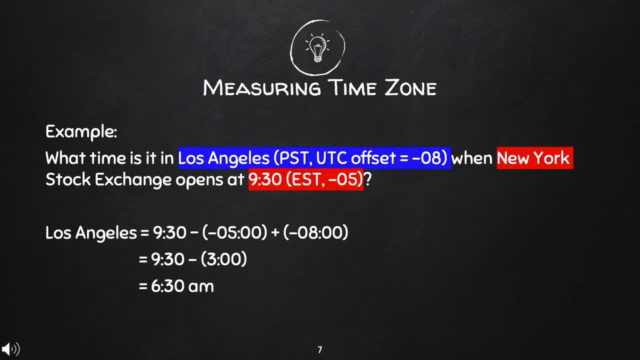 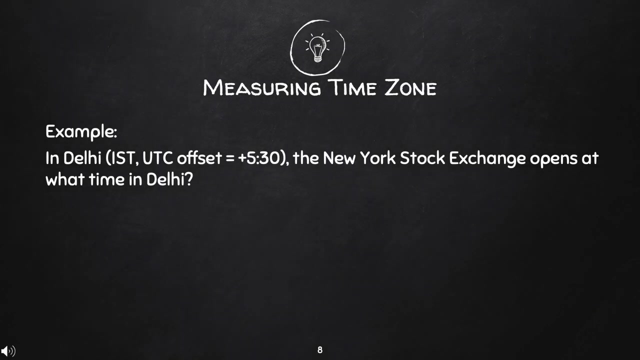 which is 5 from the UTC offset negative 8. so 8 minus 5 is 3, therefore 930 minus 3, and what remains is 630. so when the New York Stock Exchange opens at 930 in the morning, it is 6: 30 am in Los Angeles. in Delhi is the UTC offset plus 530. the 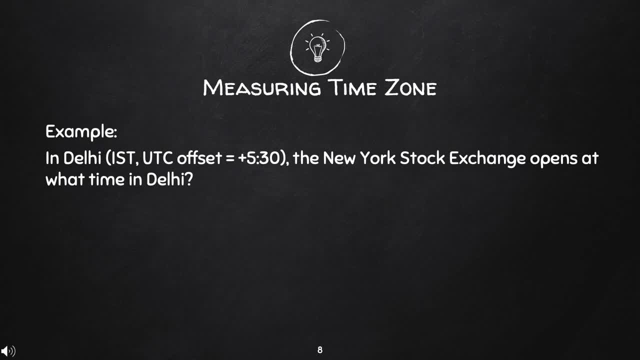 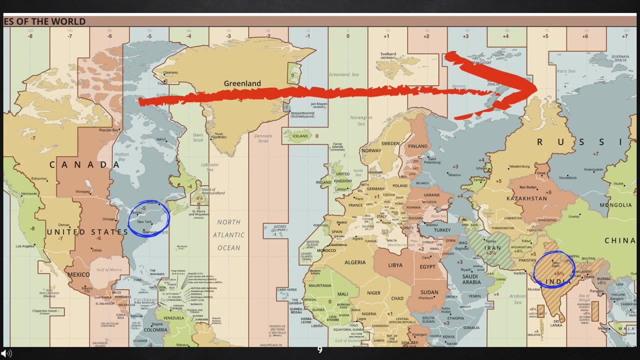 New York Stock Exchange opens. at what time in Delhi? so you see the same problem. the first problem, which is 930 in New York. what time will it be in Delhi, which has a different UTC offset? remember that here is a city in India, so look at the time zone map. we are moving from the 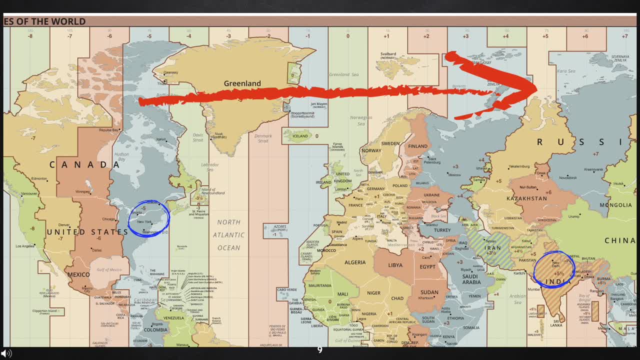 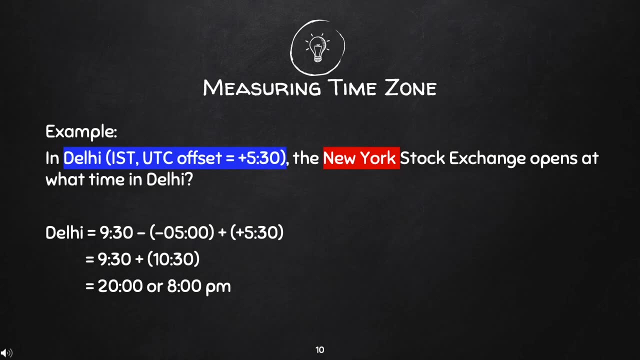 left to the right. therefore, we will use addition. you will add the UTC offsets of the two cities, which is New York and New Delhi in India. look at the problem again. highlighted in blue is Delhi, which is plus 530, and New York, which is negative 5 or minus 5. so the formula here is: Delhi, mine, equals 930 minus negative 5. 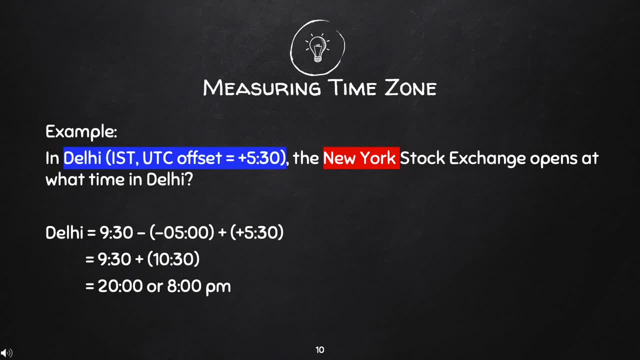 UTC offset plus 530 UTC offset. as mentioned earlier, since we are moving towards the right, we will add the time in the UTC offset. so 5 plus 530 is 1030. so 930 plus 1030 equals 20, and that is a standard time. if we convert it, it becomes 8 pm. therefore, when the New 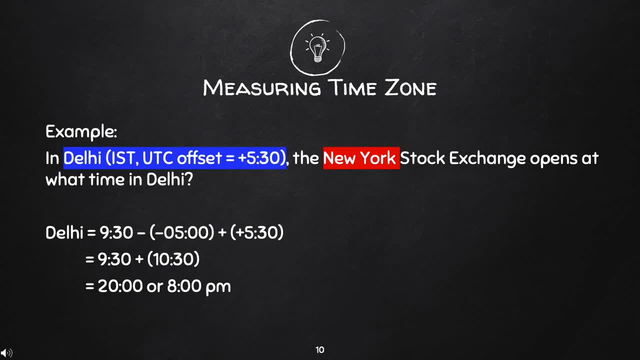 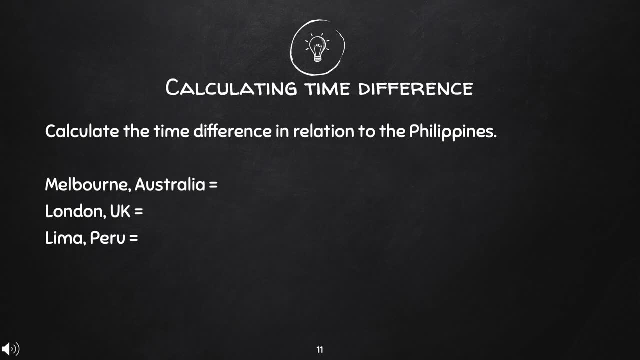 York Stock Exchange opens at 930 in the morning. it is already 8 pm in New Delhi in India. this time we will calculate the time difference between countries or cities, calculate the time difference of the following cities in relation to the Philippines. so we will calculate the time difference for Melbourne, Australia. 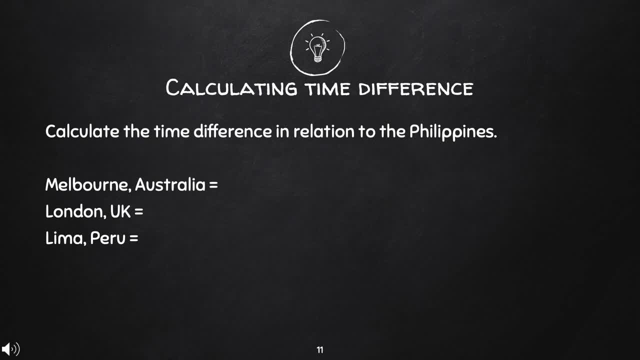 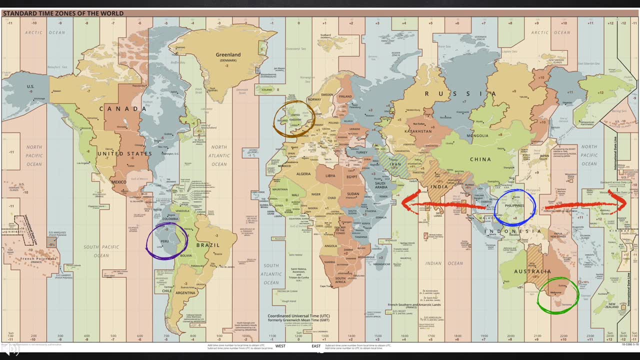 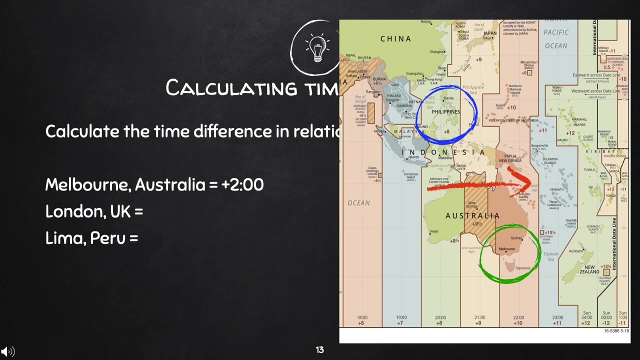 London, UK and Lima, Peru. let us look at the time zone map. in circled in blue is the Philippines, which belongs to plus 8 UTC. encircled in green is Melbourne in Australia, brown, London, UK and purple, Lima, Peru. let us first calculate the time difference between Melbourne, Australia, and the 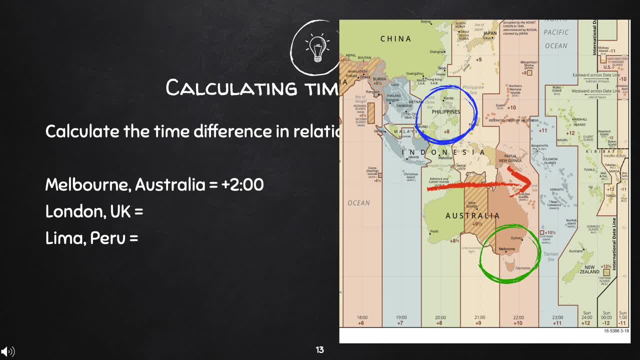 Philippines. so is Melbourne behind or ahead of the Philippines? looking at the map, Australia or Melbourne in Australia encircled in green and the Philippines encircled in blue. so we are now moving towards the right. that means Australia, the city of Melbourne in Australia, is ahead of the Philippines. it since it has. 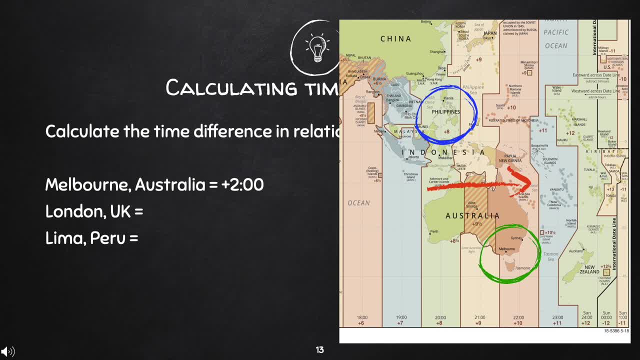 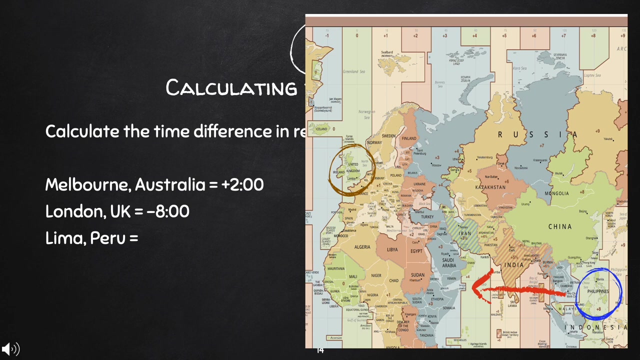 plus 10 UTC, whereas the Philippines has plus 8 UTC. so 10 minus 8 is 2. therefore, the difference between Melbourne, Australia, and the Philippines is plus 2 or 2 hours. let us now move forward to Europe. let us find the time difference between the: 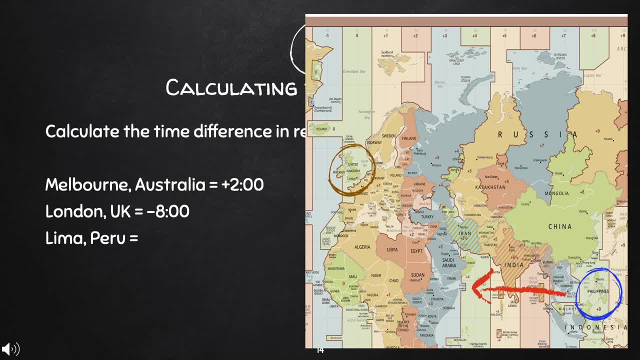 Philippines and London in UK encircled and brown is London in UK and the Philippines in blue. since we are moving towards the left, that means the Philippines is ahead of London UK. so London in UK has 0 UTC, while the Philippines has plus 8 UTC. since we are ahead, we can safely say that the difference between London